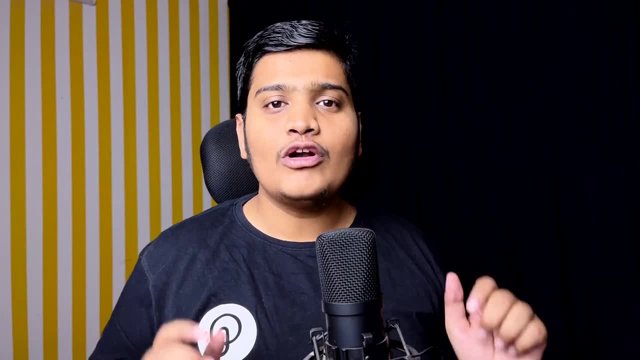 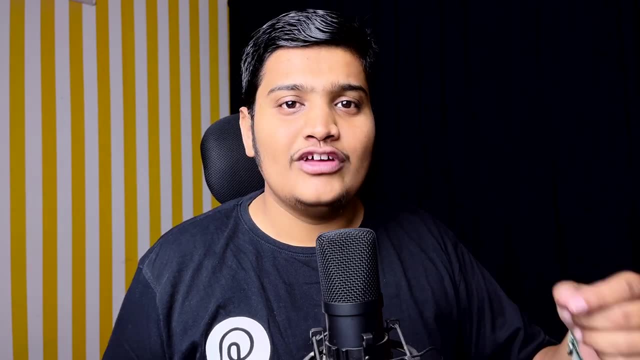 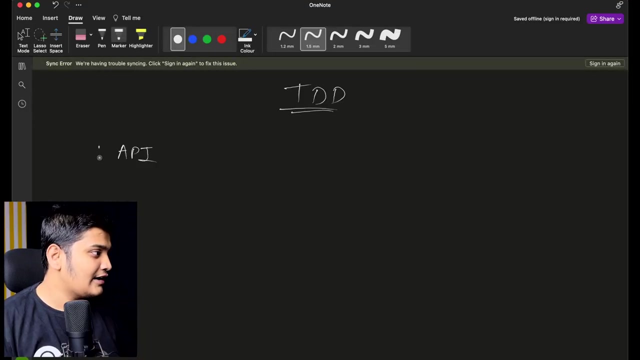 is driven by your test. Generally, what we do is we write our application, we write our APIs and all the actual code and for that actual code we write our test cases. So generally what we have seen till now is: we suppose, create an API. Suppose we created a controller For 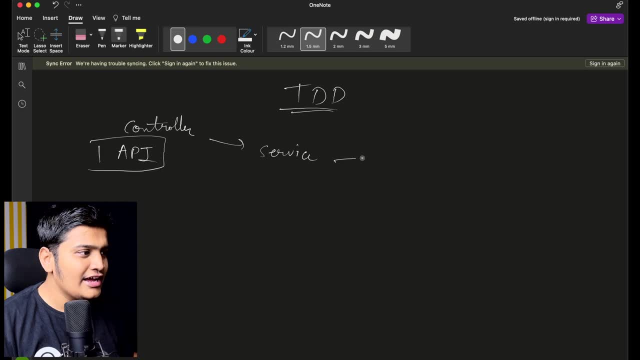 this controller. we created our service layer will write our business logic and we have a data layer where we will write the code for our database layer or your repository or whatever it is right. and for all this layer, what we do is we write our test cases. right, we write test for our controller for service. 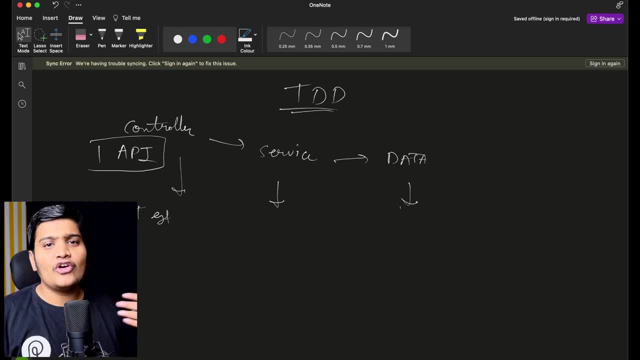 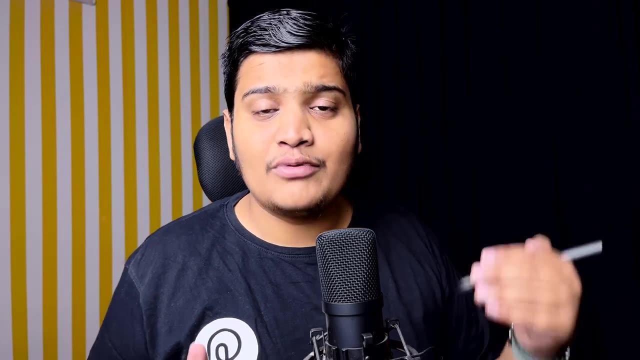 for data layer, for everything. we write our test cases and we also write our end to end test cases as well, which will cover each and everything. so this is how generally we do. now, in this scenario, what can happen is the time provided or the time given to write the. 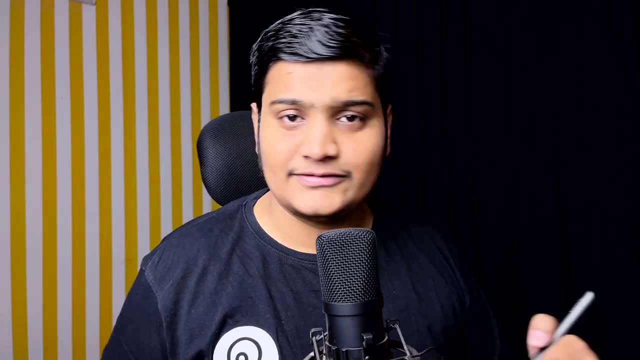 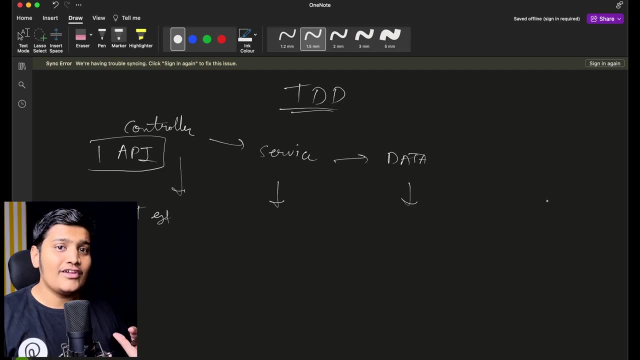 test cases would be very less than creating your features. that can happen, right, it's in any organization. So, rather than this approach, where you write test cases after your code, what we can do is to improve the quality of test, to improve the actual code, to improve the actual quality. 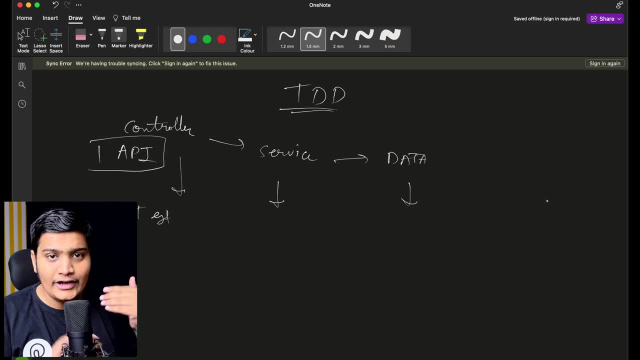 of your code. we can do TDD. that means you write your test cases first and then, on top of that, you write your actual code. ok, so let's see what it means, what is the framework for it and how we can do it. So to write your test cases. 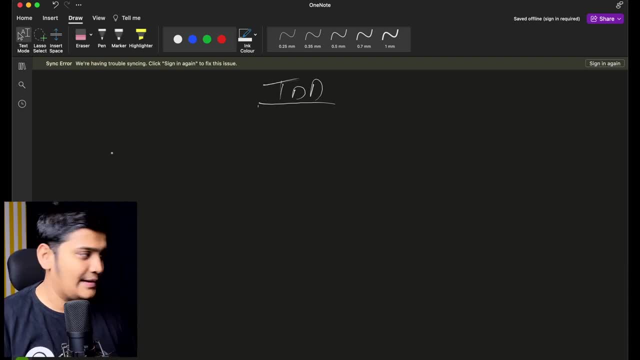 How To Make Your Test Cases Free, the tdd first. what we have to do is we have to understand four steps. okay, the steps are red, green, refactor and repeat. okay, you can call it as a framework, you can call it as a recommendation, or you can call it as a step-by-step process, but if you follow this, you will be able to write a. 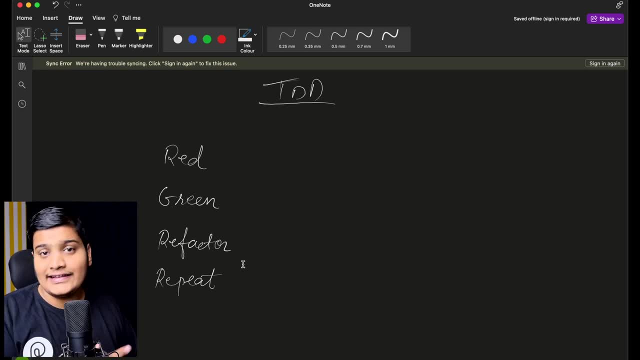 better tdd. your code will be better based on the test cases that you write, and this will help you a lot to fail. first, because you will be able to catch the bugs in your code before it go to the higher environment, so we will understand it. so what in tdd means is you write your test cases. 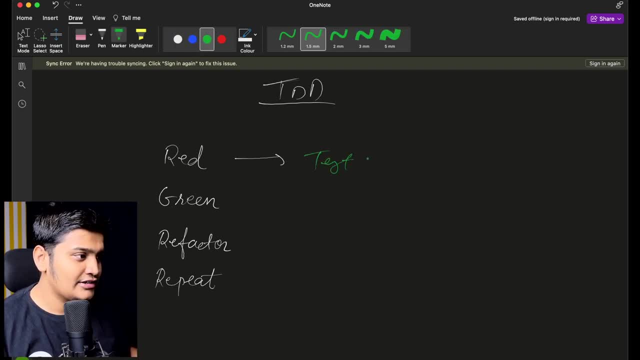 first. okay, so your test cases should be written first. before anything. you write your test cases. though it's in red, let it fail. we will write the test case first. okay, suppose i want to create one api. that api is fetching me list of photos. okay, so before i write the test case right now, 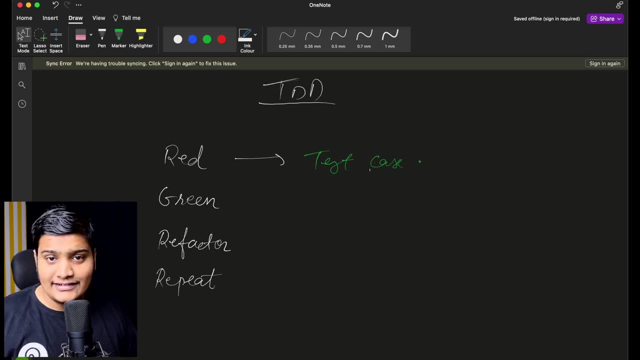 implement the list of photos API. I'll write a test case which will test that it should bring the list of photos with all the business logic details. suppose you want at least one data. you want data in this format. whatever it is, whatever the logic you need to implement, the same logic you add in your test case. so it is. 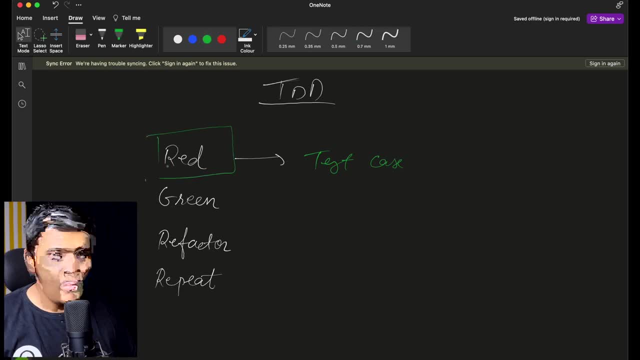 read: it's okay. okay, that's the first step. now you write your code to make this test case as green. okay, your test case is written. now you write your actual code which will make your test cases green. that means your code will be written alongside. you test your application right, so your test is. 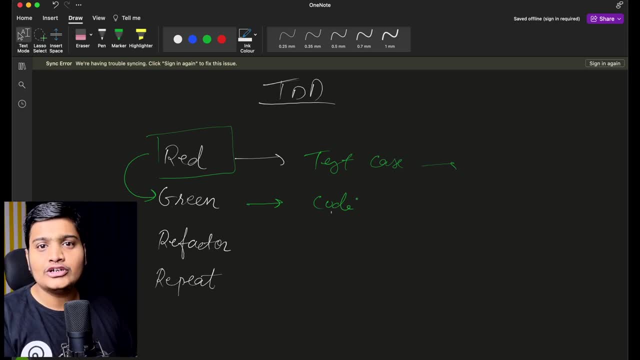 written. now you are writing code on top of that and you are also testing your application. okay, you are also testing your test cases. that means you are creating a test case and then you are converting into your code. now, at this point, your only mission is to make it green. okay, now, once that is green. 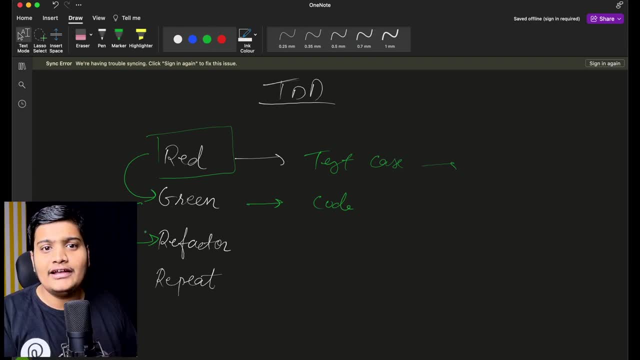 refactor your code to make it green, to make it better, to make it efficient, to make it reusable. whatever it is we have to do, do this in refactor stage. okay, this stage is to make it green. your business logic implementation, whatever it is now, make it refactor, refactor your. 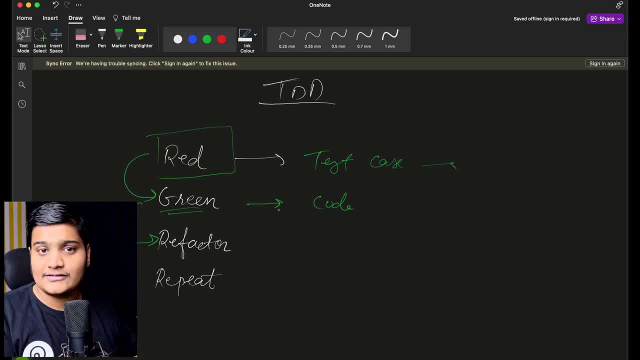 code to make it efficient and reusable and whatever it is okay, and once it is done, repeat all the steps. okay, then you again check for all the other api's, like, build your other api's with that, build the other service layer with that, and for each and everything, follow these four steps. okay, that's the basic agenda. basic. 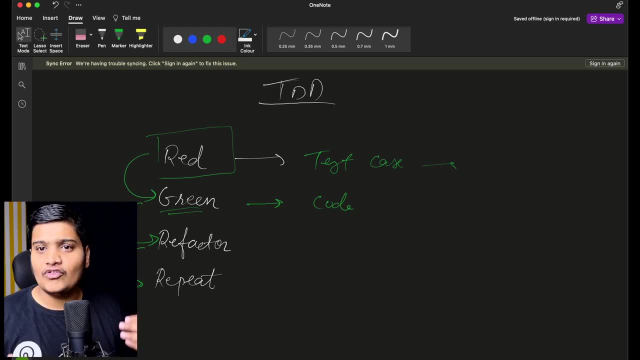 concept behind TDD. if you are following the steps, then you will be able to write your test cases efficiently and your code efficiently with very fewer bugs. okay, so this is the idea behind TDD. if there is no framework as such, this is the concept that you need to implement. okay, so we are going to implement one of 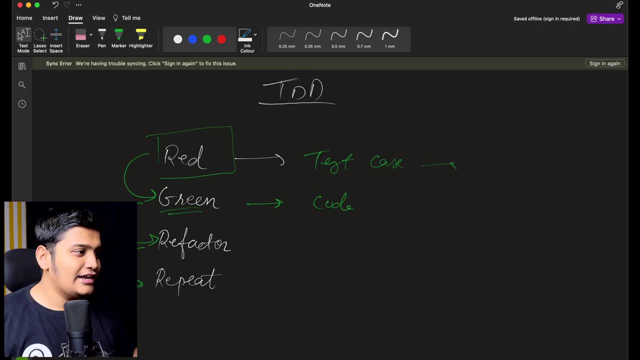 the api's with the help of this thing. okay, so let's go, we will create one test cases and, based on the test cases, we will create the api for it. okay, so let's go ahead and go to our springboard project. so we are going to create one springboard. 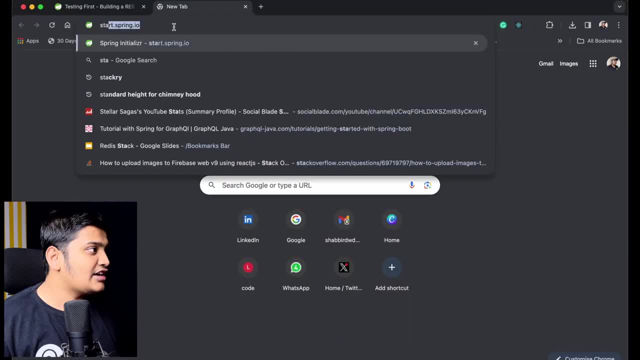 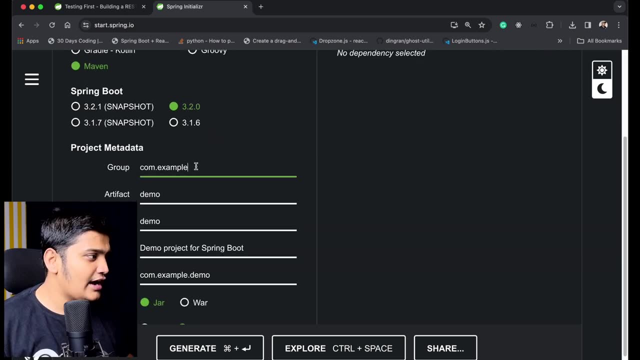 project here. so we'll go to the browser and we'll go to startspringio. so here we are going to use Java maven project, we are going to use springboard at 3.2 and you're going to say this is TDD demo. okay, and I'm going to rename. 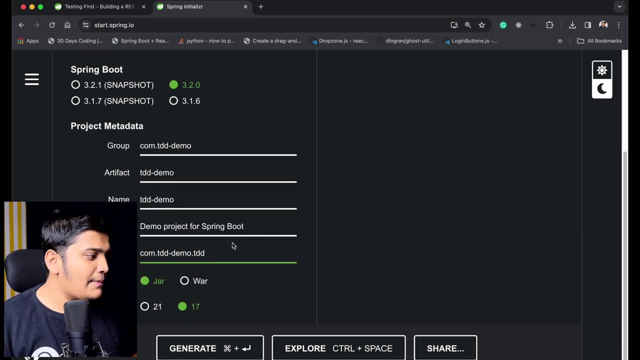 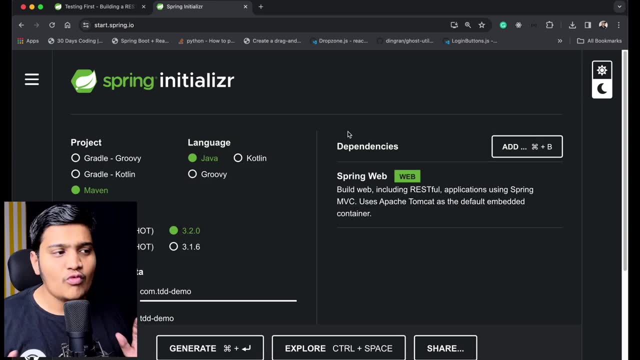 this package as TDD. okay, my packaging is jar, Java version is 17 and what I'm going to add is I'm going to add spring web dependency, because I just wanted to show you how the TDD will follow. but ideally you can add your jpa SQL, everything and you can add the test cases for all your 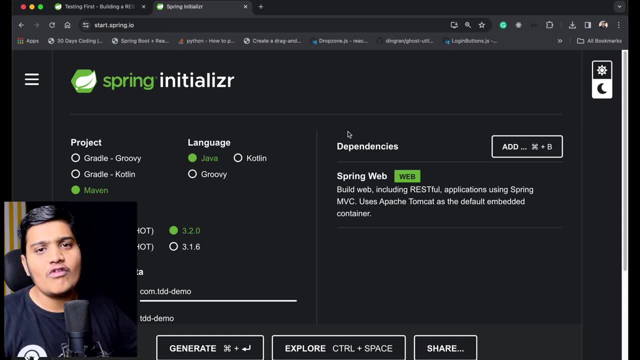 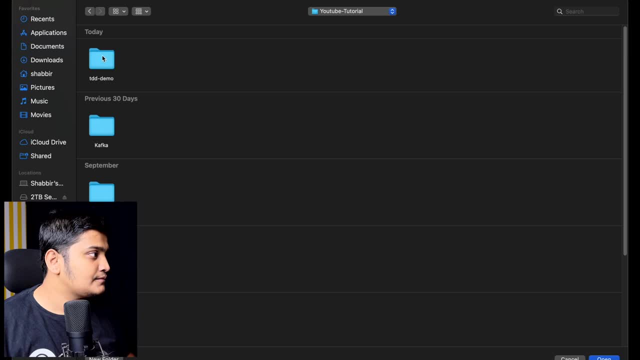 layers. okay, so let's start it with simple and, as a homework, you can build on top of it. so this is my simple project. let me just generate it and open an IntelliJ IDEA. so here you can see that I open the project. that is TDD demo. and now we have to create a TDD demo. and now we have to create a TDD demo on the project that is TDD demo. so now we have to create a TDD demo, and now we have to create a TDD demo. and now we have to create a TDD demo, and now we have to create. 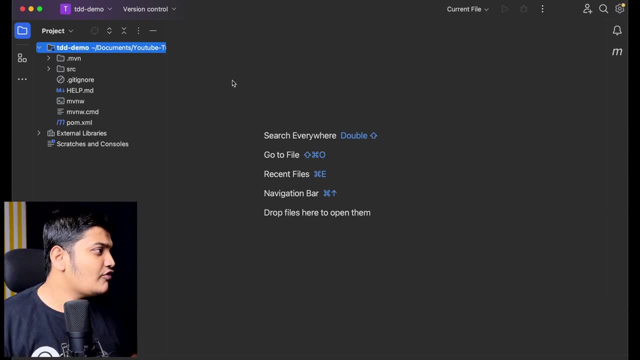 one api that will fetch me the photos. okay, simple thing. so for that we will write test case first and based on that we will write our code. so this is my simple application here you can see that this is my main package, where my actual code would be, and this is my test package, where my 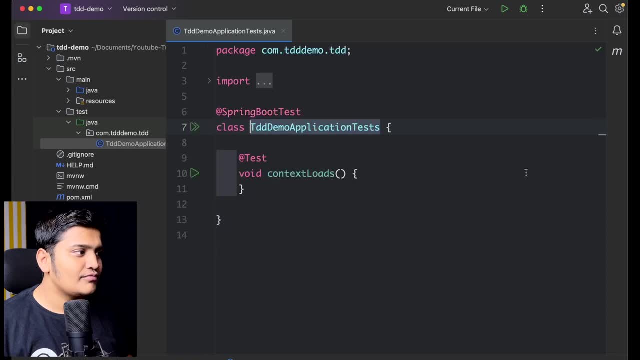 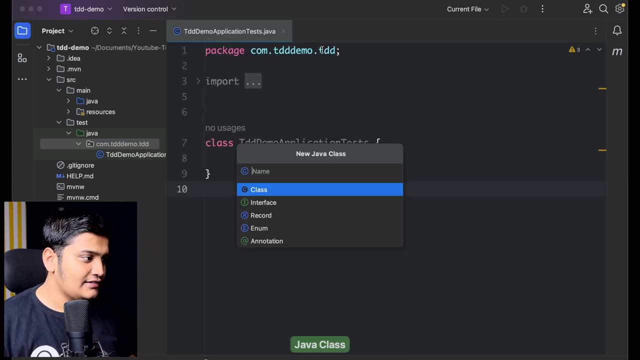 test cases would be, and there is already one test case available. okay, so what i'll do? i just remove this, okay, and what i'll do? i'll create a test case, java class, and i'll just name controller. within controller package, i will create photo controller test. okay, this is the class that i'm 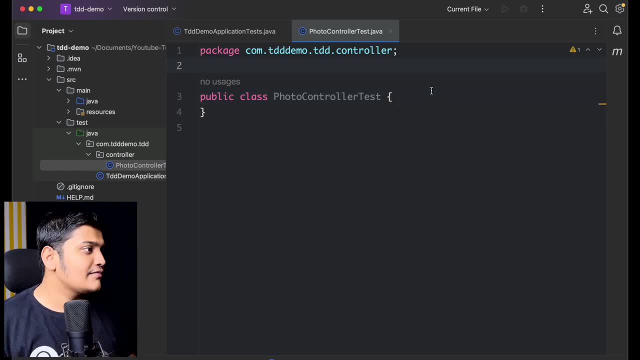 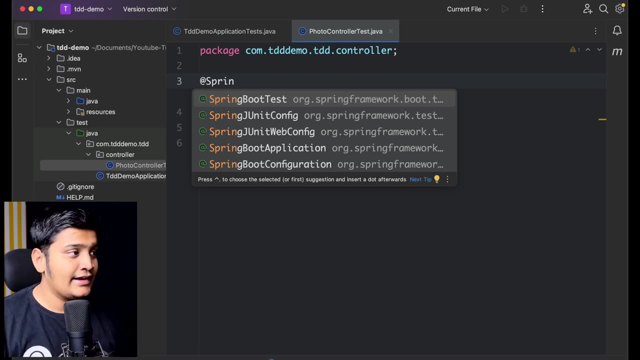 creating now. this is what i want to write now. ideally, i can write at the right spring boot test. that will give all the configurations for me. but i do not want everything. i do not want the entire context here. right, i just want to test this class, so we will just add the configuration accordingly. 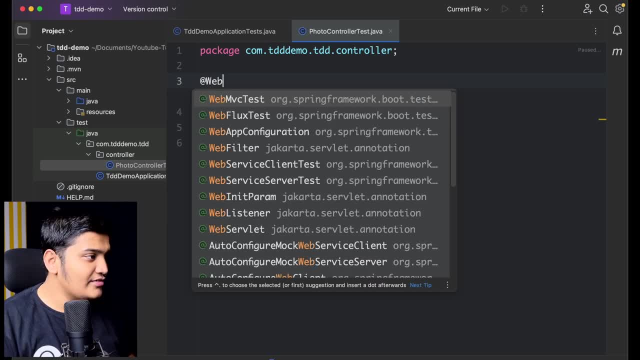 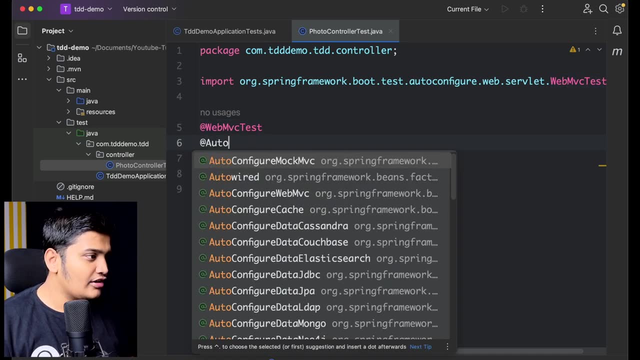 so what i'll do? i will just tell that i want web mvc test. so i'll just tell that i want web mvc test and i'll add the configuration accordingly, just annotate with this and i will auto configure this. so i'll just mention auto configure mock. 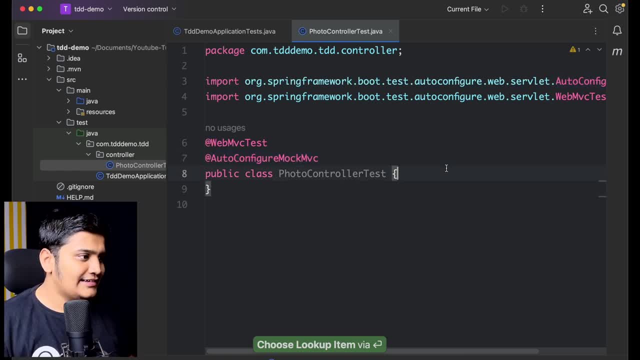 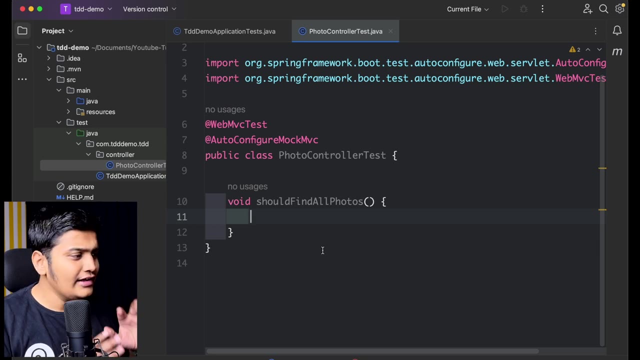 mvc. okay, now let's write a test case here. so i'm writing test case: void should find all photos. okay, i am mentioning that whenever i hit an api, i should get all the photos available. okay, this is what i want to do and for this, what i'll do, i'll mention this is a test case. 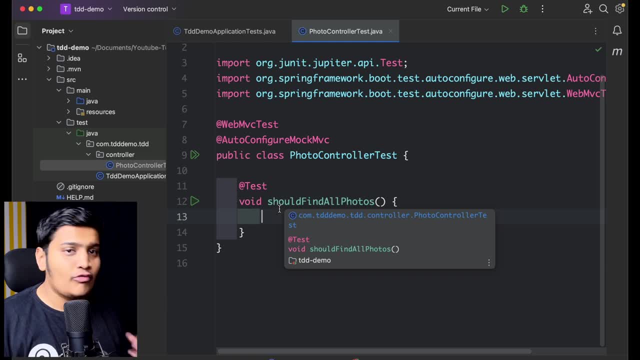 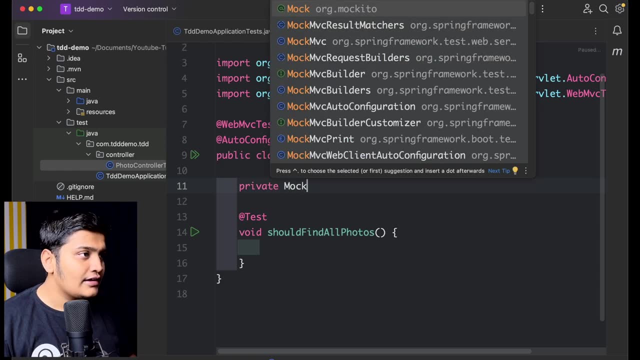 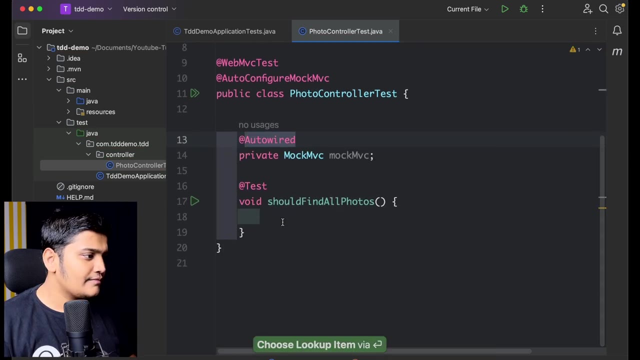 okay, now to perform the api call here. what i need: i need mock mvc object, right? so i'll just add the mock mvc object- private mock mvc- and i am going to auto wire it. okay, so here i can write: mock mvc dot. perform mock mvc. 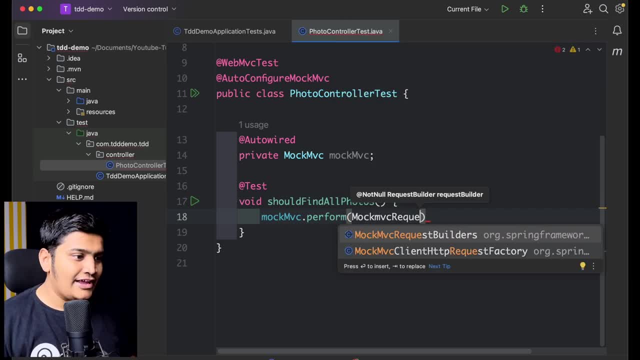 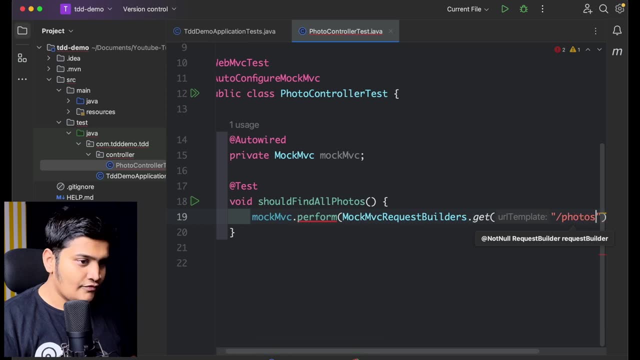 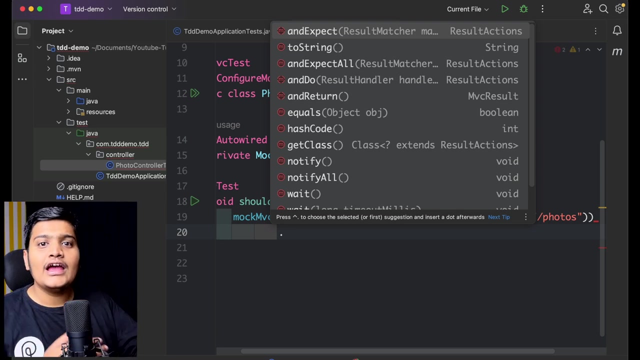 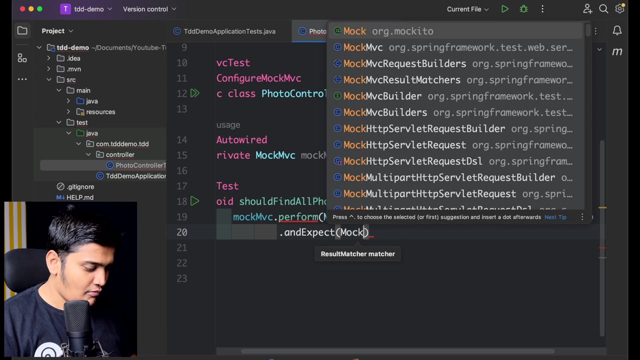 request: builders dot get. and i'm going to give my uri that is, photos. this is what i want to call and what i'm going to expect in return. so whenever i hit this api i need 200 okay status. that means my api call is successful. right, i can mention and expect: mock mvc result: matchers dot. status: dot is okay. this. 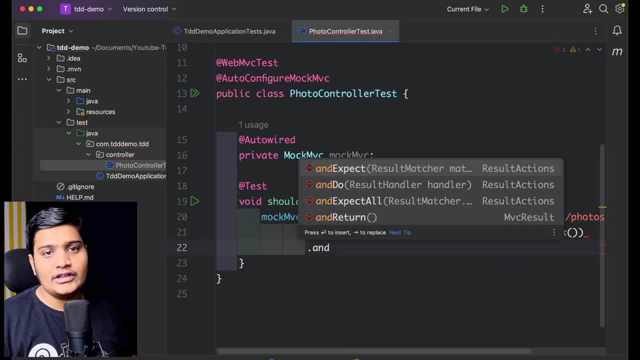 is one thing i'm expecting here. and i'm expecting one more thing: that i should get at least three records. okay, not, at least i should get three records. that's what i'm expecting, because possibly i am passing three records and i have three records in my database. that's what i'm. 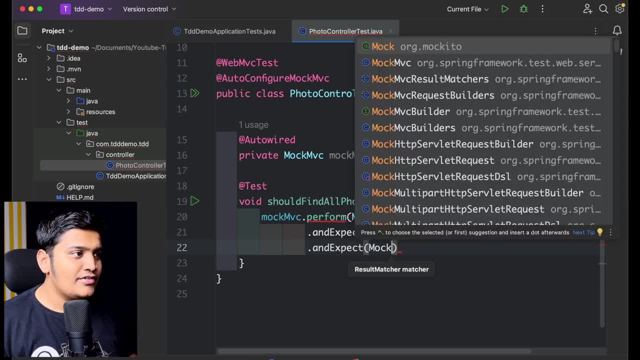 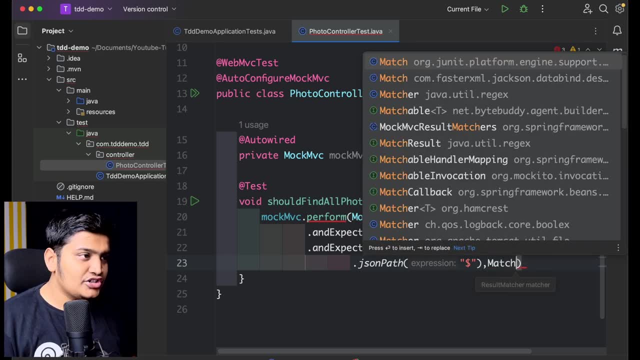 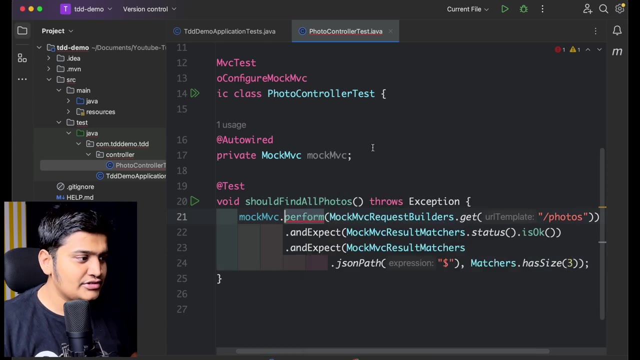 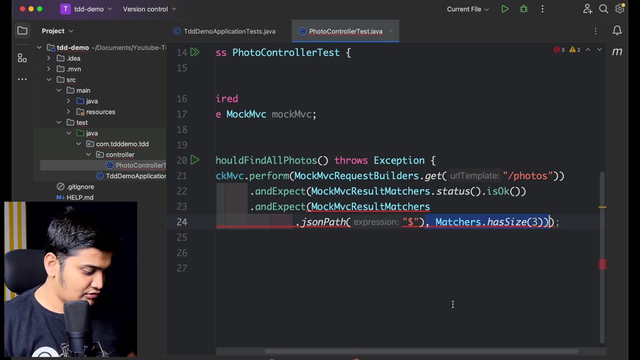 assuming okay. so i'm adding and expect mock mvc result: matchers dot json path and i'm taking the root element here and i'm telling matchers dot has size of three. okay, this perform will throw the exception, so let me just add it here. getting some error? let me just resolve it. i think i gave it outside, so it should be. 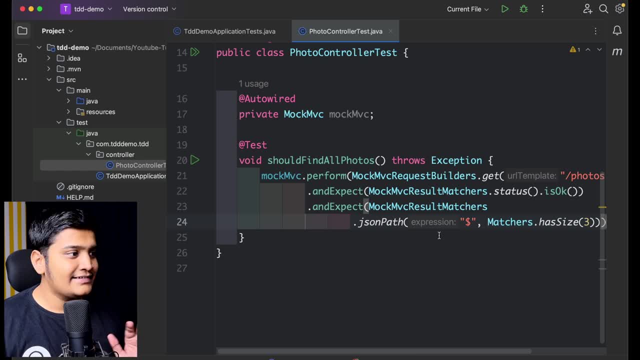 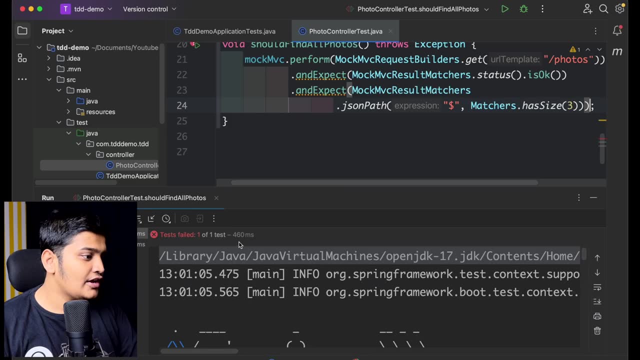 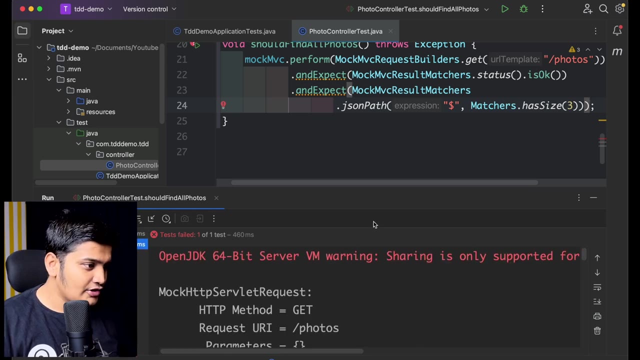 okay. so this is done. so simple. this is my test case. now if i run this, you can see that it is red. so our first step is done: that build a test case which is red. it's okay. so if i go here- okay, you can see that. what it is telling? that we are getting 404 here. that means it. 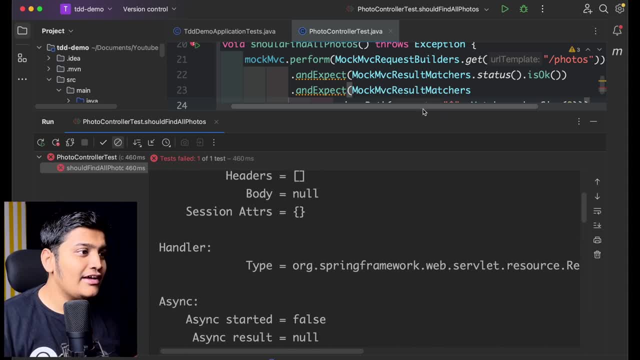 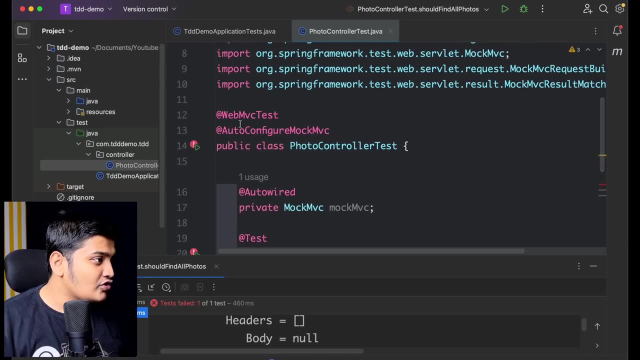 is not able to find the test case. so i'm going to go here and i'm going to go to the test case and i'm going to run the entire test case like this. so now it's running already. okay, now this is a little bit frightening, right? so we're gonna just take a less fast look from this, so we're just gonna. 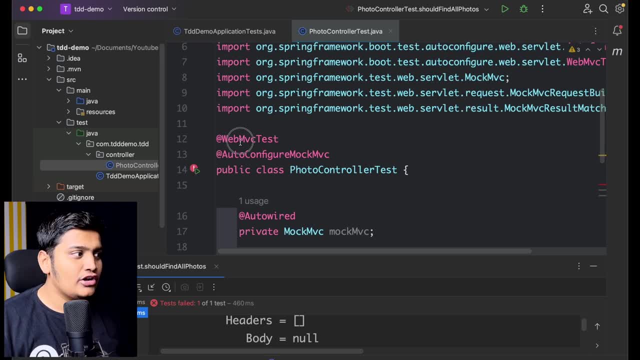 break it down right here. so again, it is the test case that is on the sce. built alsoَ and new is the source of theitutional error option here. so that's, that's a non-�. we're going to save this bar, all right, and now i'm going to send my test case from my sce tool at the sceiles. so let me. go into remote and i'm going to set up a touch lens in the whereas. alright, so now, if i'm going to save this, i'm going to write down what is my basl and hl to get it. this is, let me spin it, and i'm getting 3 records. so 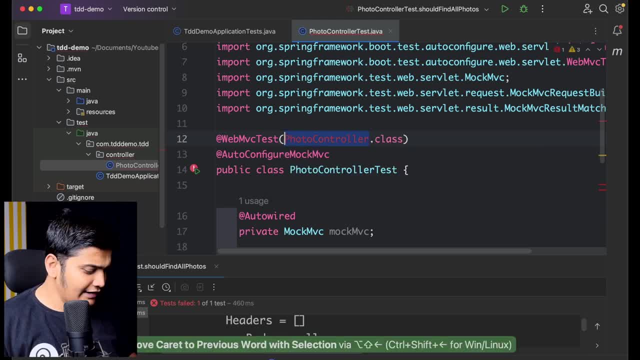 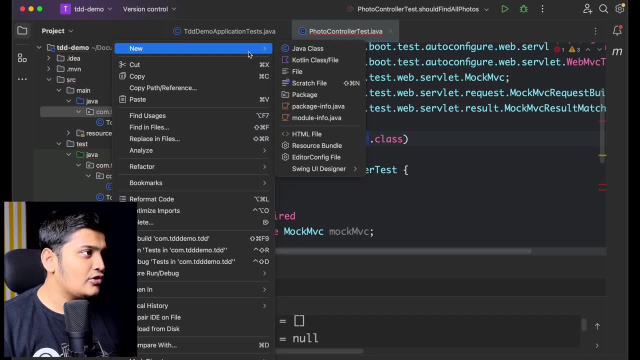 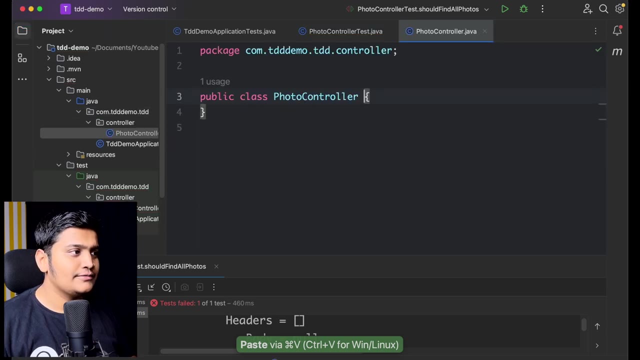 dot class. now this class is not available, right? so i need to create this class. so what i'll do? i'll go to my main and there i'll create the class. so i'll go to new java class. i'll mention controller package. within that controller package, i need photo controller. okay, now, if i come here, 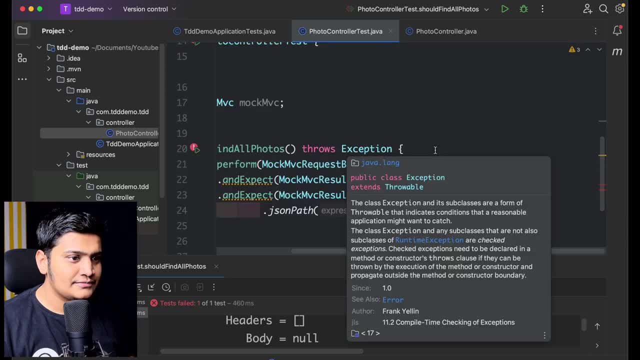 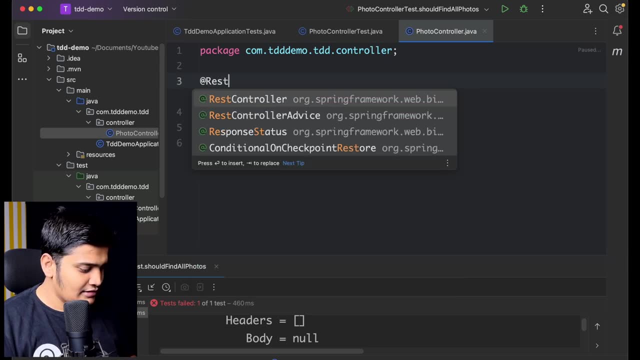 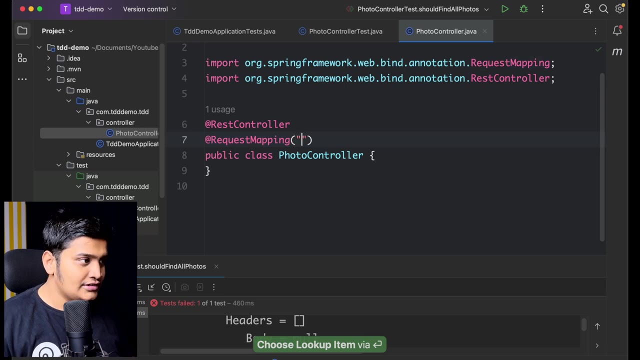 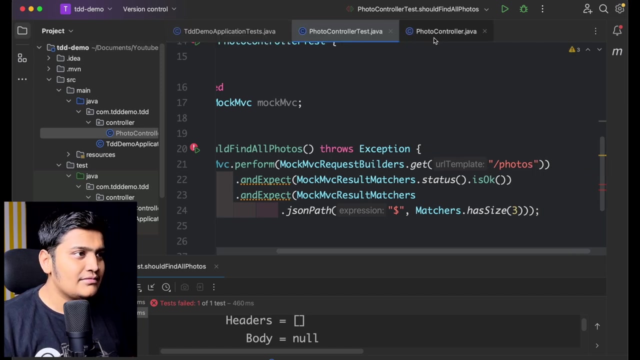 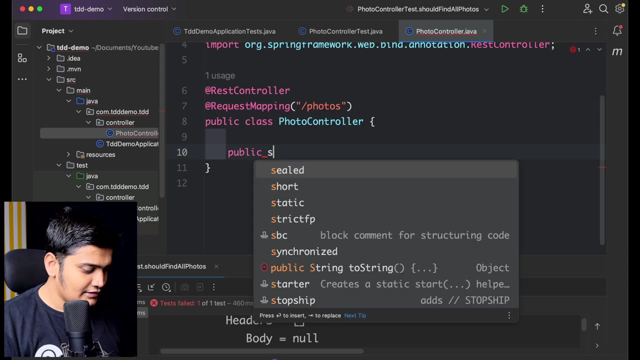 you can see that that error has been solved here. okay, and now this particular class has to be rest controller. okay, and it should support request mapping to slash photos. okay, because this is what we are building: the api: slash photos. so you can see that particular thing has been done. now i need to have one api. so what i'll do? i'll just create public string. 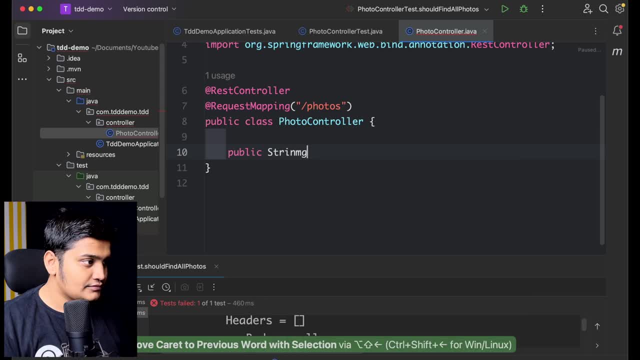 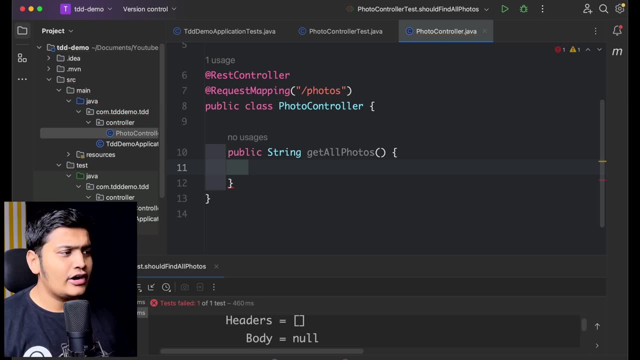 get all photos. okay, this is the method that i am preparing. you can call it get photos or get all photos, doesn't matter. okay, and this is my get mapping and i'm telling: return blank as of now. okay, so you can see that my api is done now. okay, so from here i'll be able to call this. so let's. 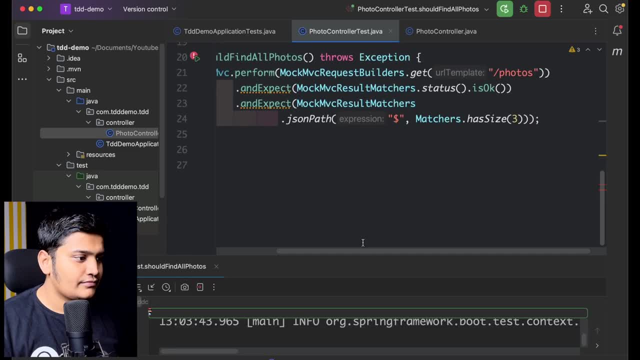 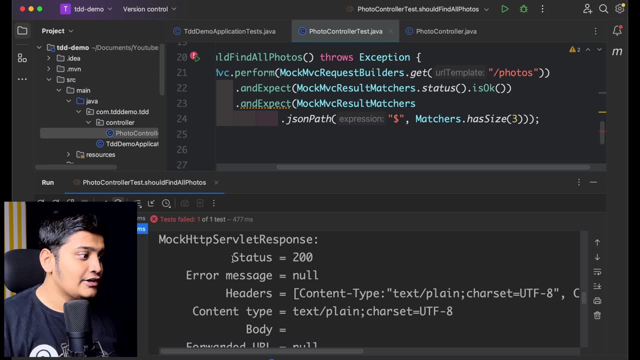 test this so you can see that still we are getting. let's see what happened. and okay, one thing is there that you can see: we got status 200. that means the api which we are not able to find. that is resolved now. there we have another error. so 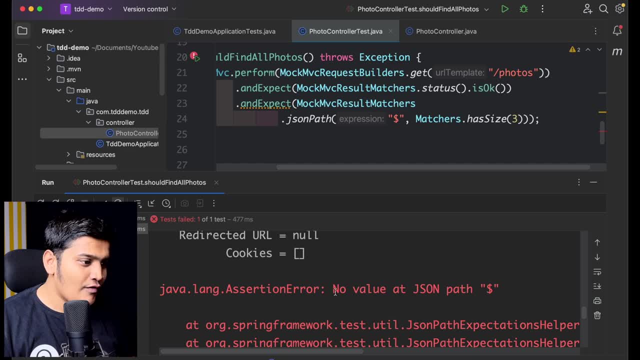 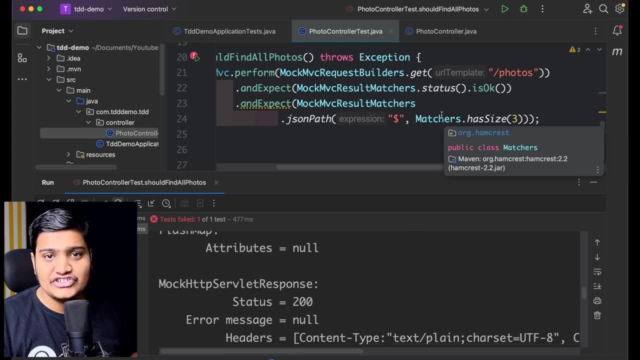 let's try to check that. what is the error? okay, so no values as json path: dollar. so that means we are not able to or we are not sending. you can see we are not sending anything as json here, right? so what we have to do is we have to first send the json data. right, what we are going to send. 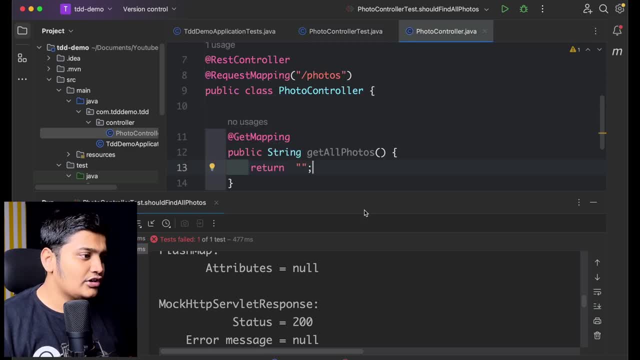 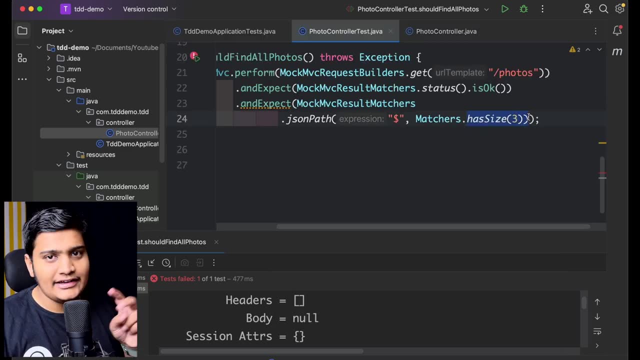 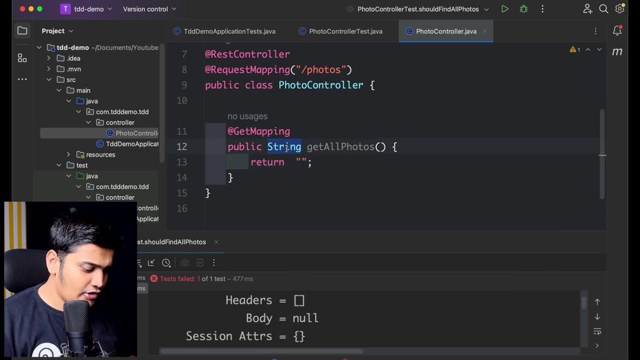 okay, that particular thing we have to build. so, within this photos controller, what i'll do is, rather than returning string, because i am expecting here three records, right, that means i need to send a list. okay, so here also, rather than sending a string, i need to send a list. right, so what i can do, i can send a list of what i can create a model. 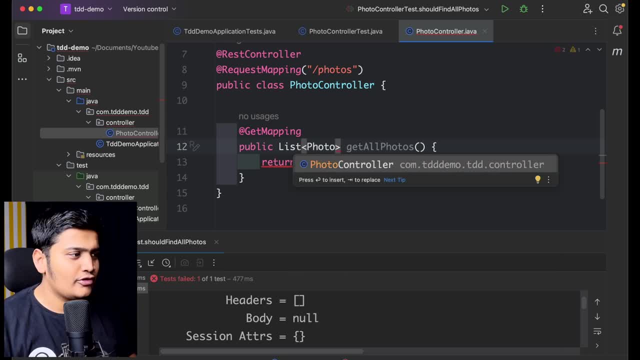 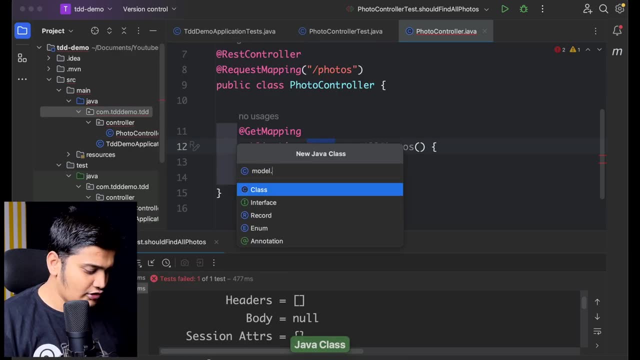 generally we create the models, right? so suppose i'm creating a photo here. okay, so this photo is not available, so i need to create it, so let me just create it. i'll create a new java class and i'll say model dot photo and this is what i'm going to create as a record here. okay, so i just created a record of photo and 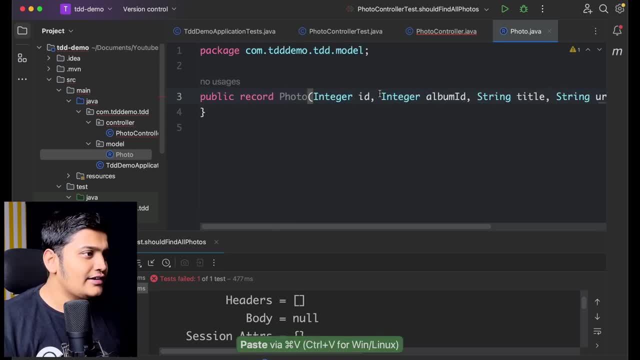 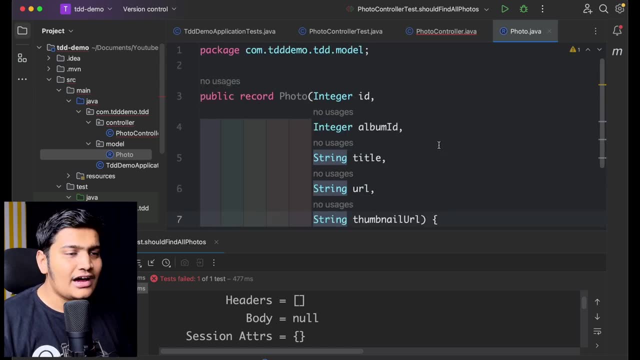 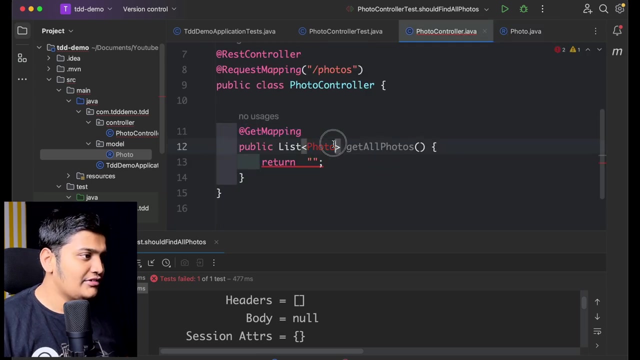 within this photo i am adding some of the parameters. okay, so you can see. i added integer id, album id, title url and thumbnail url. okay, so these are the data. these are the input that i'm giving, so this will be the data type. so if i go here to photo controller, let me just import photo now. 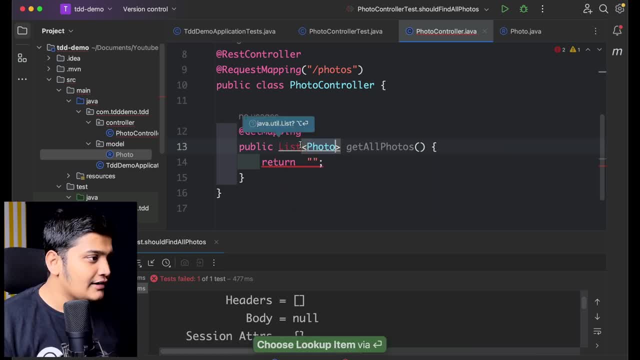 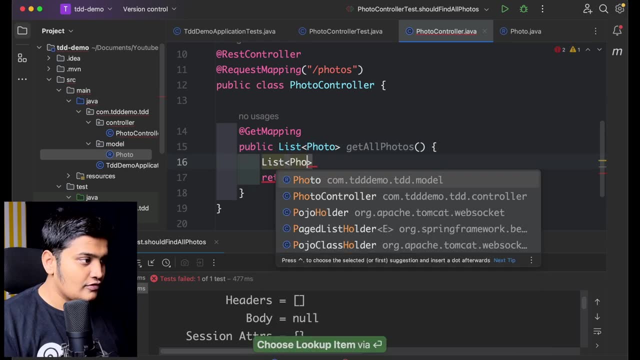 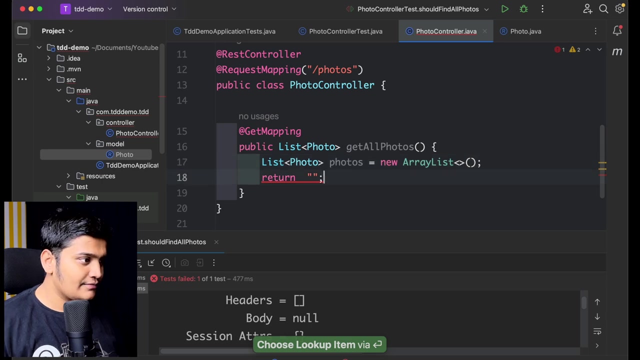 because i have created a photo. now, okay, let me just add the list as well, and here i can send the list back. so if i create the object of list of photo as photos equals to new error list, okay, i can send the photos back. okay, now, if i run this, i should still get the error because i have still 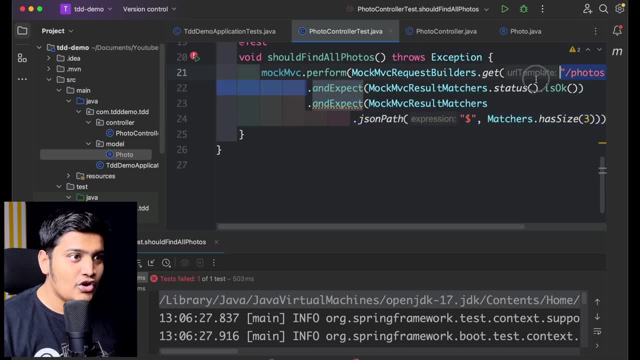 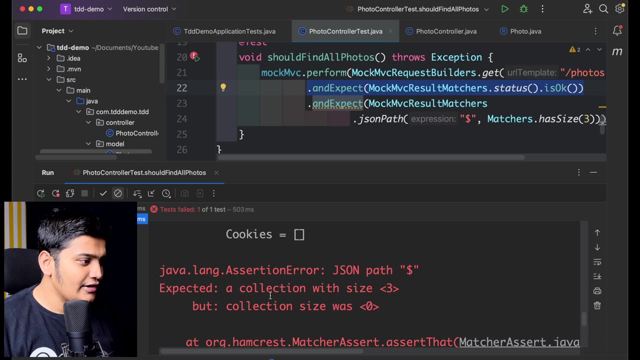 not suffered. suffice this one. i suffice this one. okay that my epi is there, which will going to send a be okay result, but i'm not getting three records here. so if i still see, okay, i have still the same issue. okay, expected a collection of size three, but the collection size. 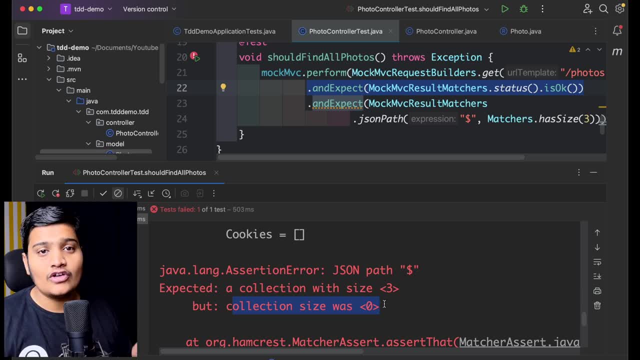 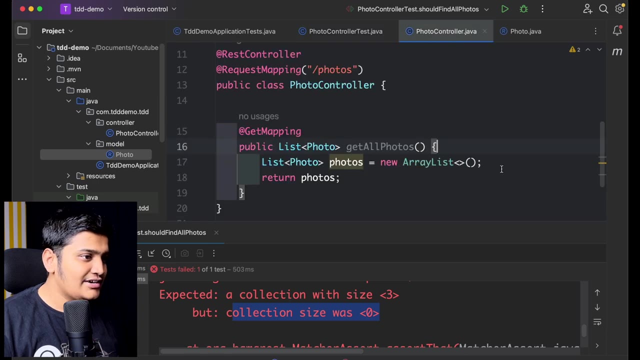 was zero. so now you can see that that error is also gone. where it was saying that it's not a particular token, it's not able to particularly identify the json, right? so you can see that how we are solving this. now let's go and add some data here. so what i'm trying to do is i'm adding. 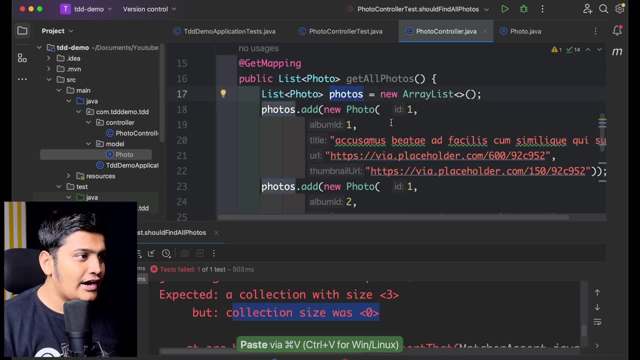 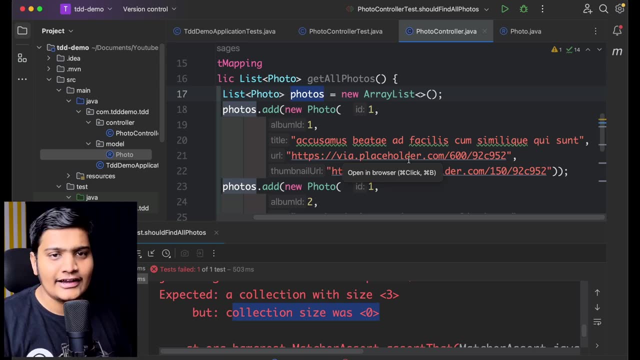 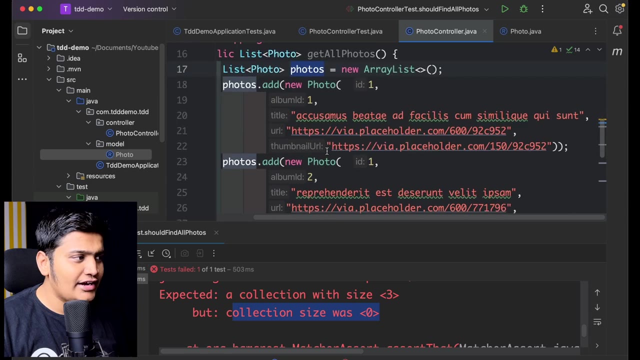 some data. so within photos object, photosad, i am creating a new photo where i'm passing the data. this data i have taken from json placeholder so you can take any data from there. from there i have taken the photos object. you can create any other object as well. okay, so i just pass bunch of data. 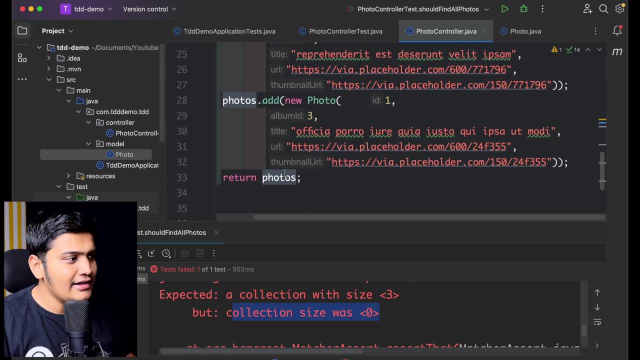 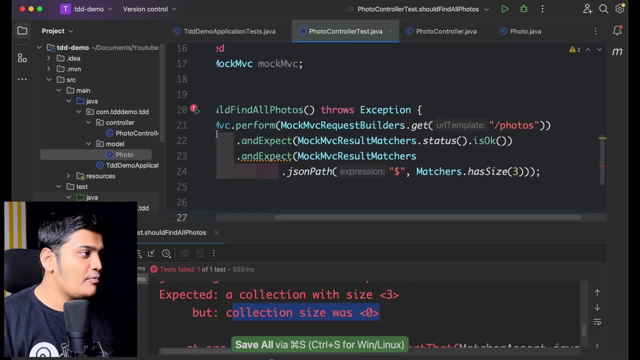 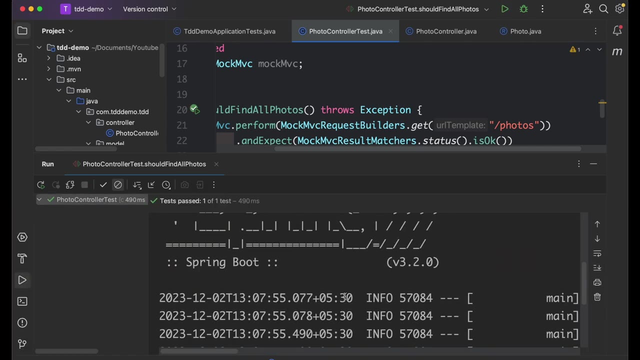 here and accordingly this data should be populated and should return back. so i was expecting three records. so i have done three records here, okay, so once this is done, if i go back and if i read on the test case here, you can see that my test case is passed right. so that means, whatever the test case, that 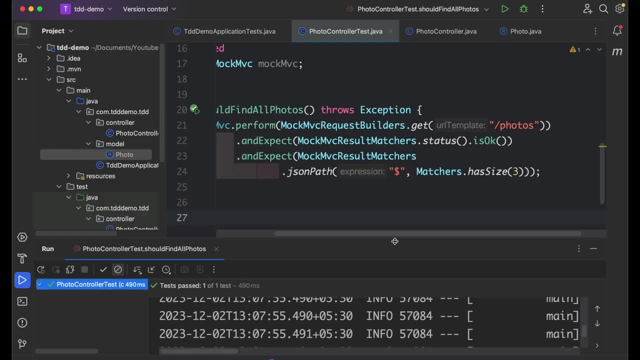 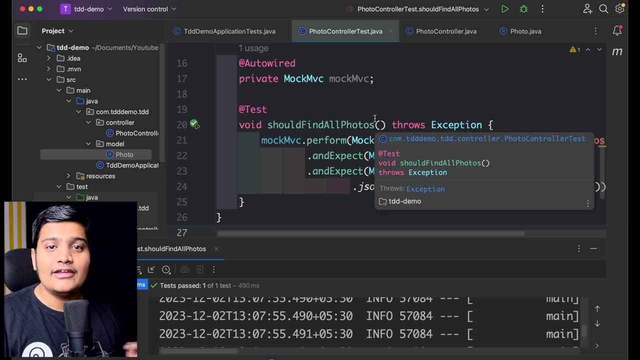 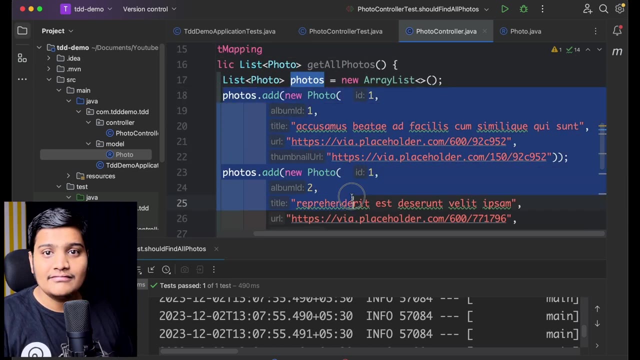 i had written all the business logic there. accordingly, my code has been working right, so now what i can do is the next third step is refactor. so are there any improvements that i can do? are there any improvements that i can do in code? yes, so this is the all idea about how you write the tdd and how you write the. 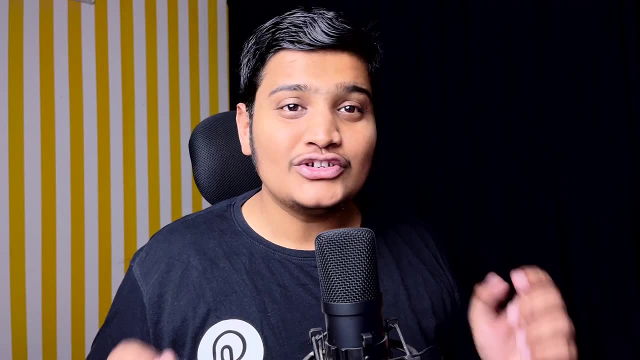 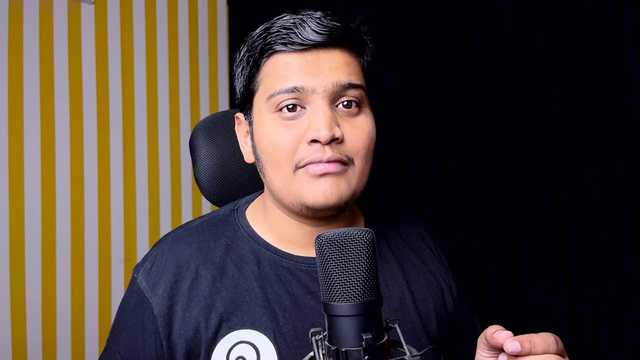 how to improve the code quality and test quality. So this was all about the TDD which I wanted to share with you. It's really easy to implement. You can see, this is just a concept that you need to think in mind, So it's not about just completely shifting to another framework. 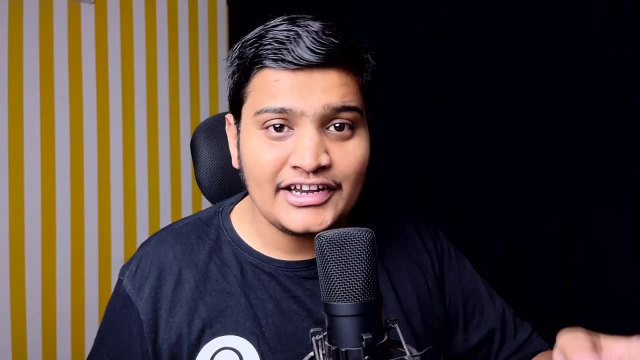 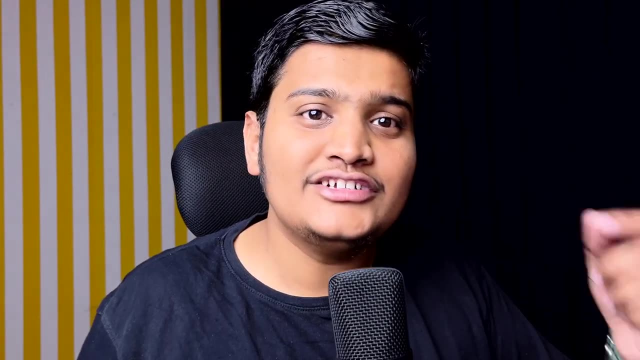 It's just like shifting your mindset. rather than just starting your implementation, your actual code, think about writing your test case first and accordingly build on top of it. So it will just improve a lot better your code quality and your test quality and it will benefit you. 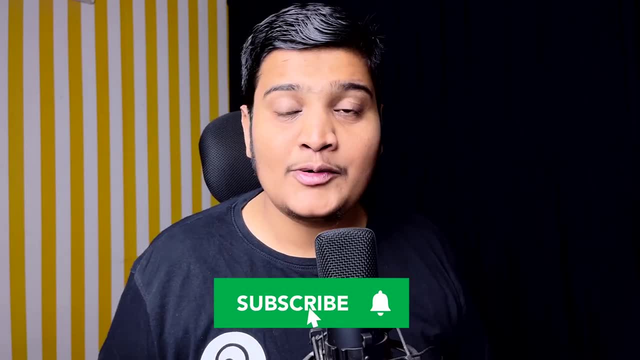 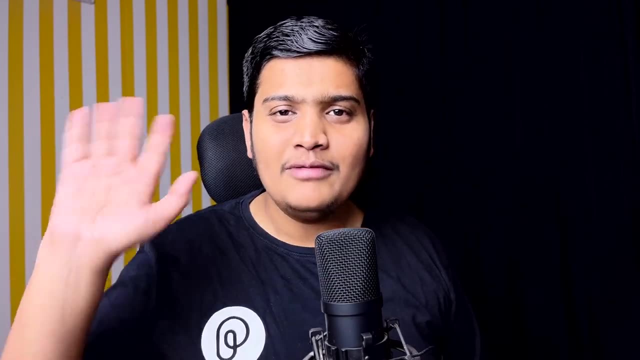 So that's it in this video. If you like this video, give us a thumbs up and subscribe to my channel for the upcoming videos. You can also click on join button to join my channel. I will see you in the next video. till then, happy coding. Bye.